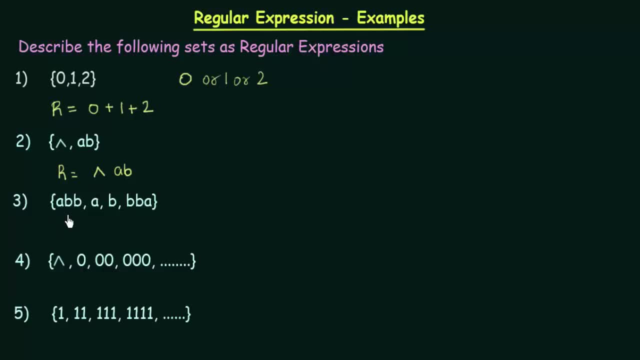 Alright, so I hope that was clear. So let's come to the third one. In the third one we have the symbols ABBA, AB and BBA, So this means that it can be anything like ABB OR A OR B OR BBA. 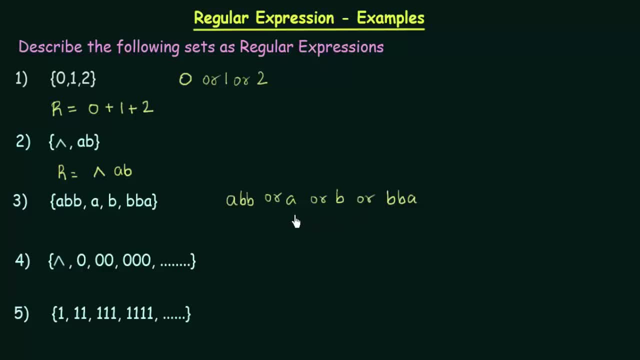 So any of these symbols can be Present in the set Or a language that contains this. Any of these symbols will be accepted. So how do we write the regular expression? It is very simple, Just write, since it is a OR here. 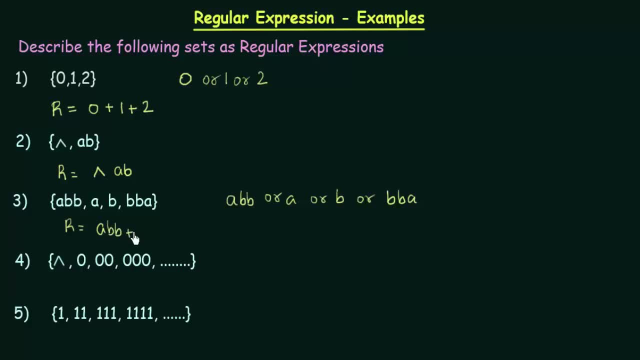 We just have to use the plus symbol ABBA OR A OR B OR BBA. So this is how you can write the regular expression for this set. Alright, Now let's come to the fourth one. 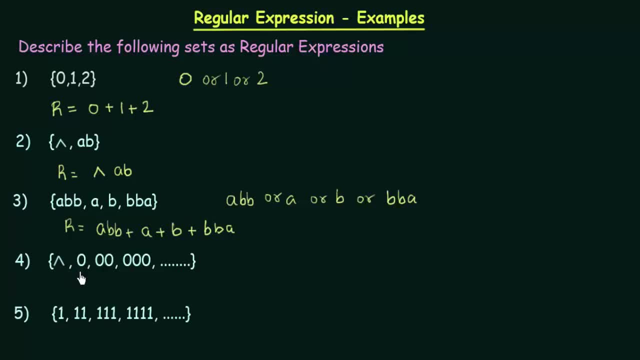 So here we see the empty symbol, then 0,, 00,, 000 and so on. So what is this? I have already explained this in the last lecture, If you remember. if you look carefully, you find that these are any strings that can be formed by using the 0 symbol. 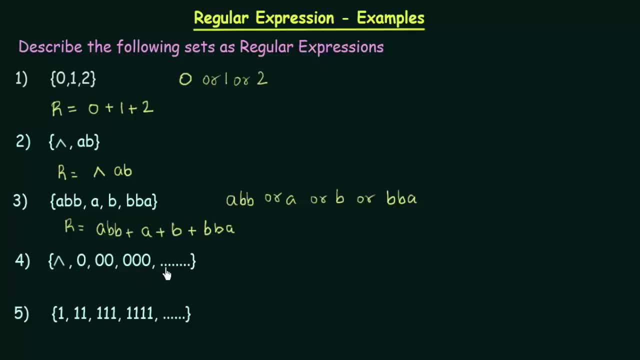 0,, 00,, 000 or any more symbols that can be formed by putting together any number of zeros that you want. So all the strings that can be formed using 0, along with the empty symbol. it denotes the closure of 0.. 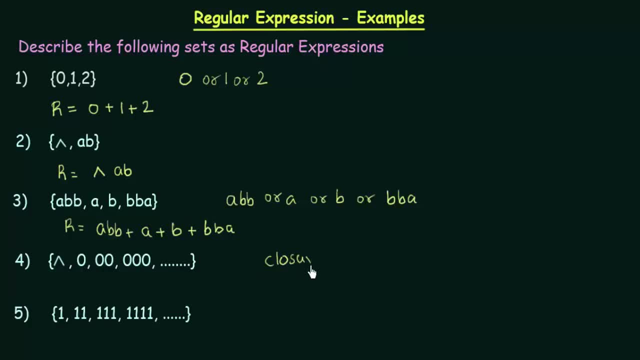 So this is the closure. This is the closure of 0.. So how do we denote closure? I have already explained This can be denoted by R equal to 0. closure When you give a star mark or an asterisk mark as a superscript. 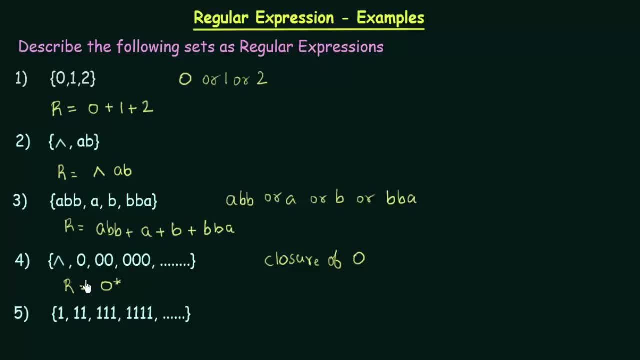 it denotes the closure of that symbol. So this is 0- closure. Alright, So let's come to the last one. Here we have 1, 11, 111,, 1111, and so on, So this also means any strings that can be formed by using this symbol 1..